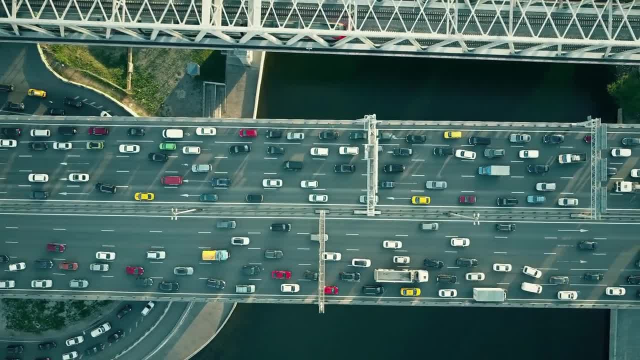 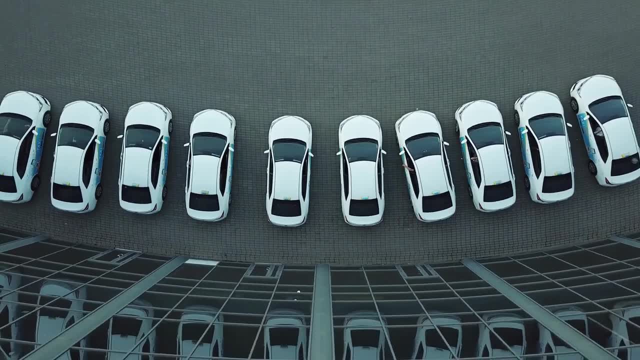 our society is run. We believe that people should be able to get where they need without having to rely on cars or public transport systems that cause so much harm to residents who live near them due to air pollution and noise pollution from engines, not only while driving, but also. 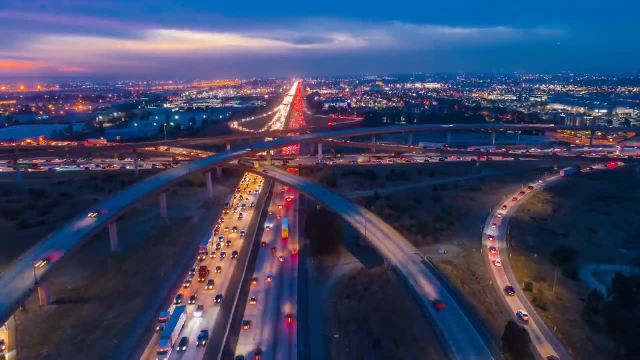 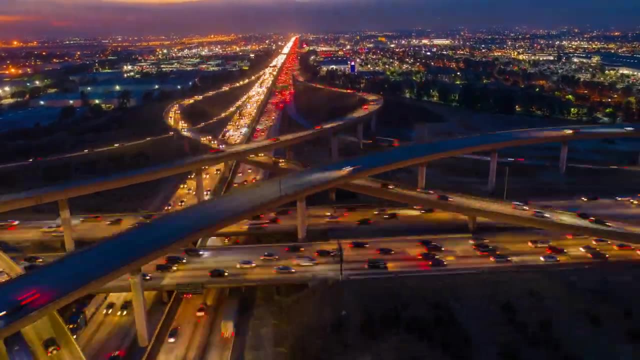 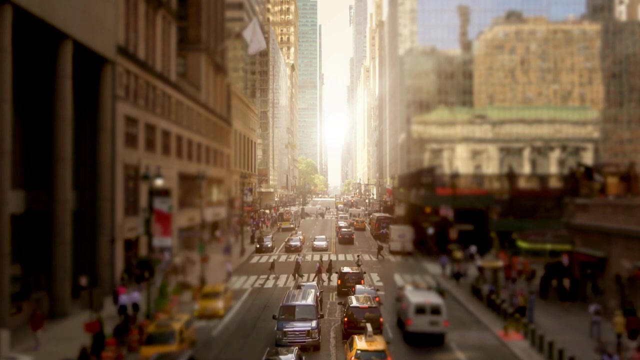 when idling at bus stops or train stations. This convenience can come with significant consequences. Smog has been proven by scientists all over the globe as being bad for human health because it causes respiratory diseases like asthma. The future of sustainable transportation: The future of sustainable transportation is: 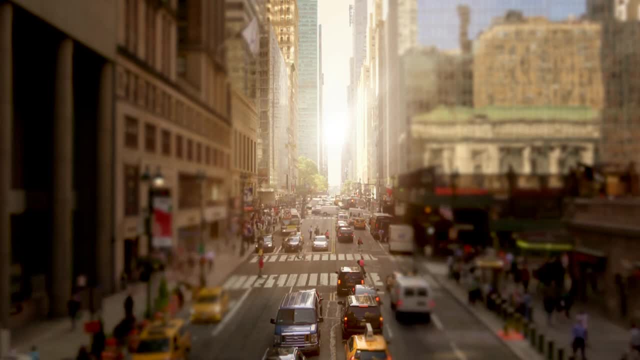 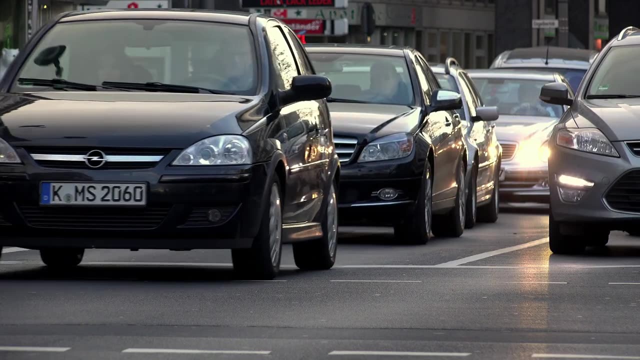 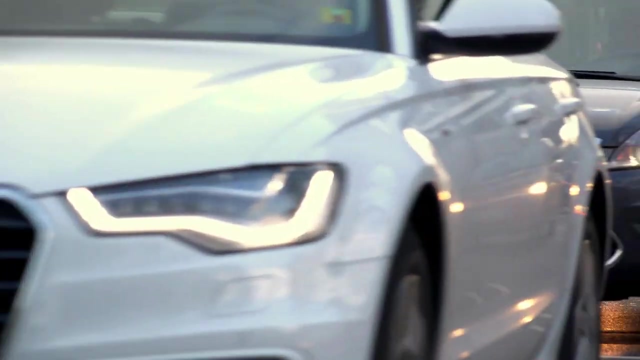 very promising Sustainable transport solutions for the future have been demonstrated by the United States with several initiatives and innovations, such as new bike lanes in Copenhagen that are designed to protect cyclists from poor weather conditions and accidents. Other examples include Bikeshare programs, which offer affordable rates across major 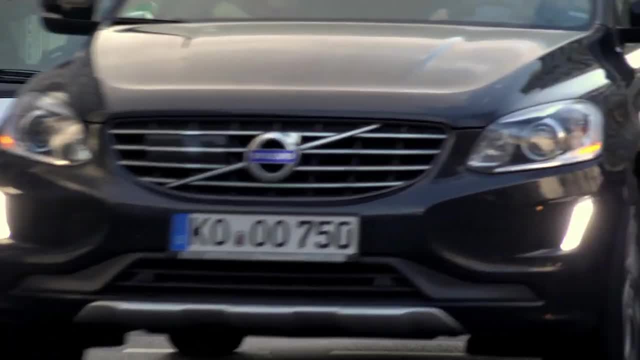 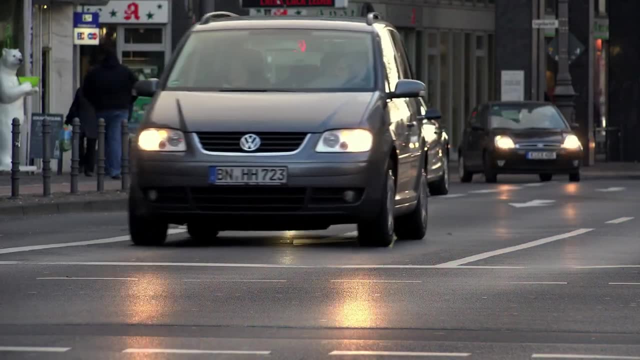 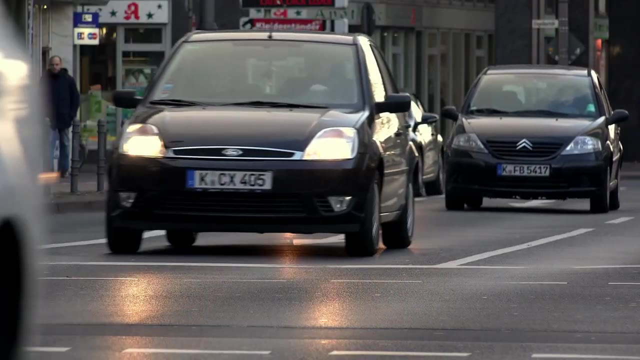 North American cities like New York City, Washington DC, Montreal or Chicago. In these programs, people can find bikes at their convenience 24 hours a day, on any street corner where there's an available docking station nearby. There are also electric cars. Bikeshare and Conleaf use zero-emission technology so they don't release harmful gases into our 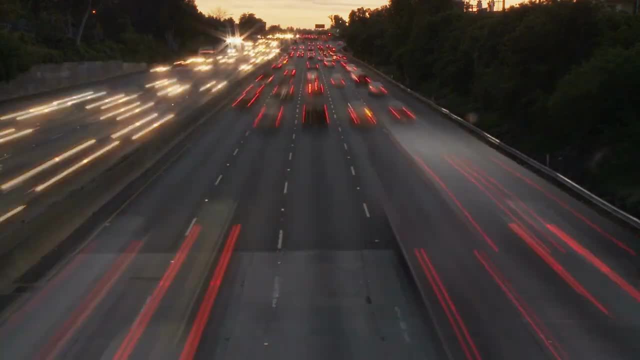 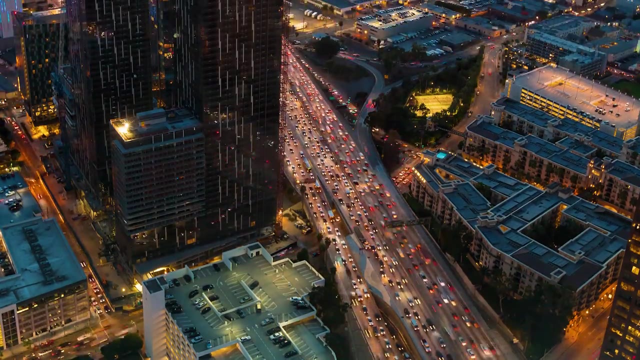 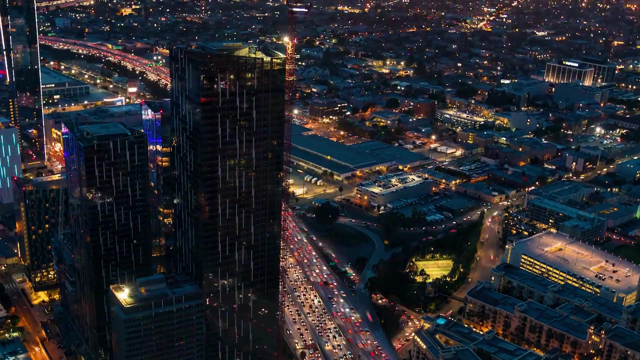 atmosphere, without considering how much CO carat gas emissions contribute to the environment. that is harmful to our health and the environment. The future of sustainable transportation is in electric cars, bikes, carpools or public transit. These are all excellent alternatives that will help us keep moving faster without harming. 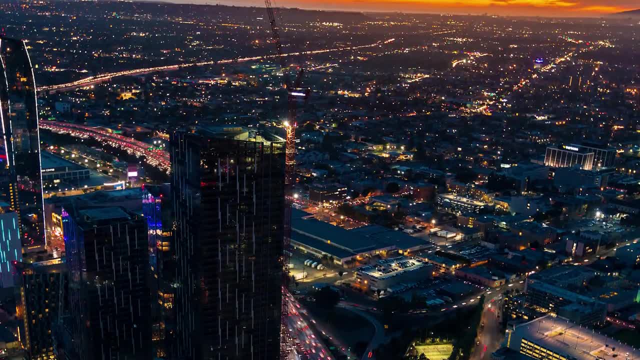 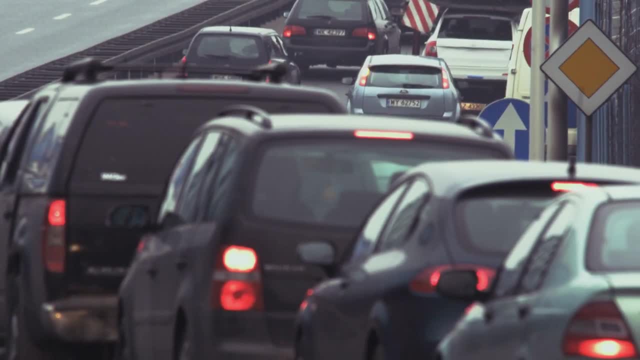 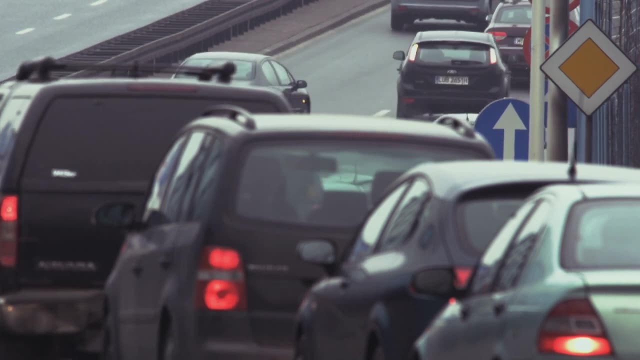 the Earth's resources. We can make more social by improving community spaces with pedestrian-friendly features for parks and sidewalks, For example. we can create new parks and sidewalks for people to visit instead of just walking through on their way somewhere else. As we learn about how technology has changed many aspects of our lives- new inventions, 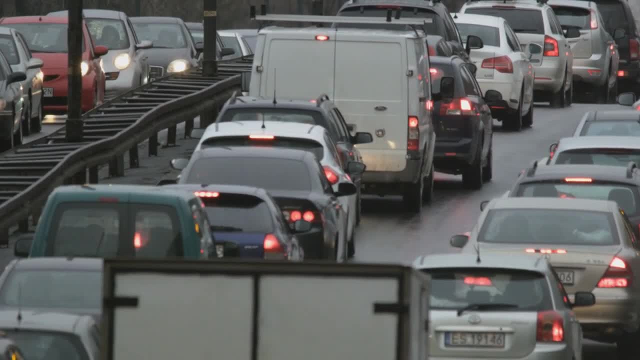 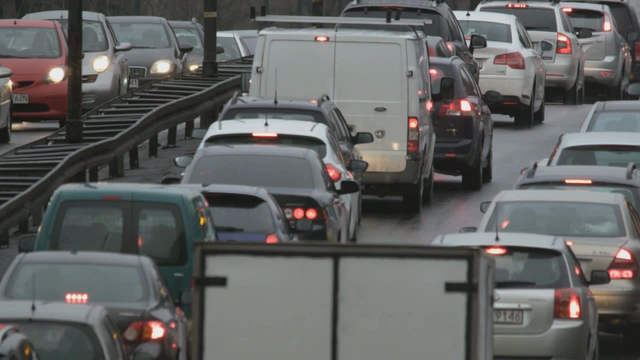 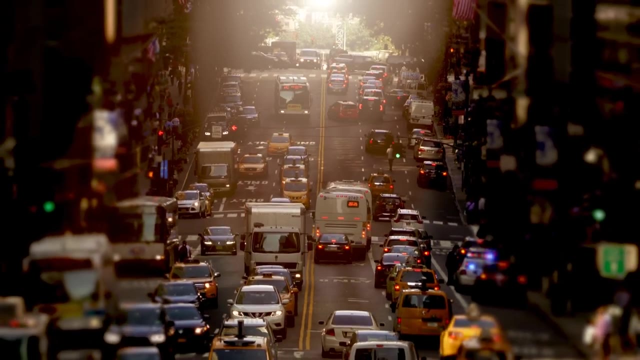 are being introduced every day, which offer innovative ways for commuters to travel, while preserving what makes cities so attractive – convenience and diversity. Benefits of Sustainable Transportation. Sustainable transport packaging has many advantages, including reduced impact on the environment. You can also save money and avoid the risk of having a vehicle accident or breaking down. 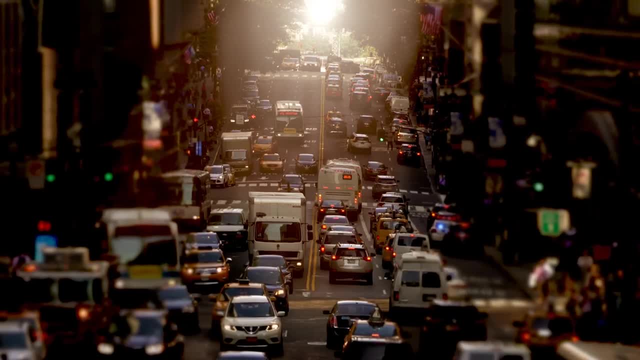 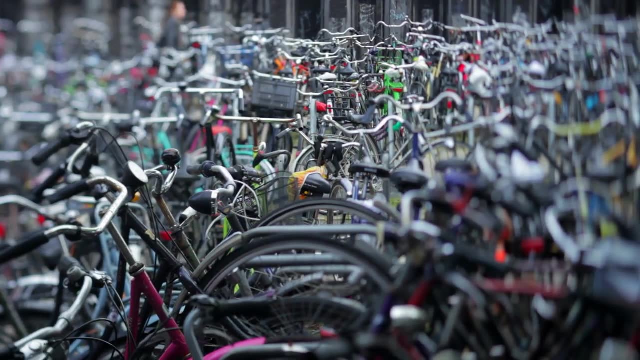 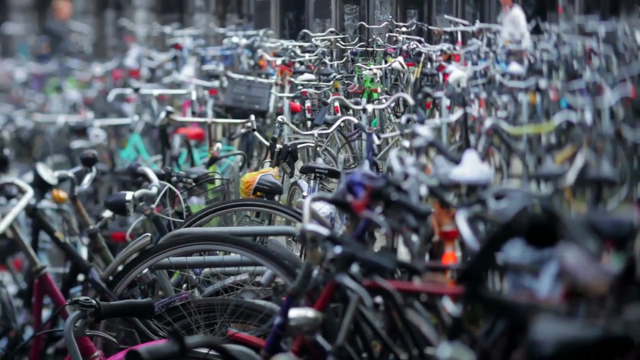 in remote areas. A sustainable transport delivery offers many benefits, with some being greater than others, depending on what you need as an individual. A few of these benefits include: 1. Reducing Your Carbon Footprint. One significant advantage is that by using sustainable transportation packaging, you can reduce your impact on the environment. 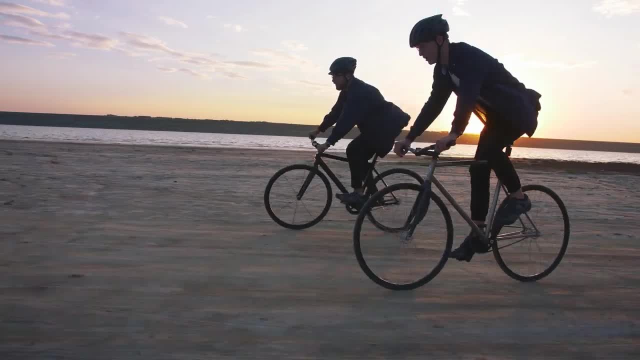 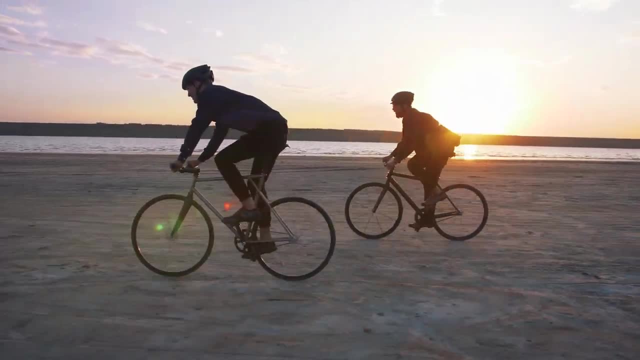 while reducing your carbon emissions and saving money at the same time. 2. Avoiding Vehicle Breakdowns and Accidents. Transport packages have also been proven to be more reliable when it comes to resisting damage from collisions because they don't require any fuel for operation. 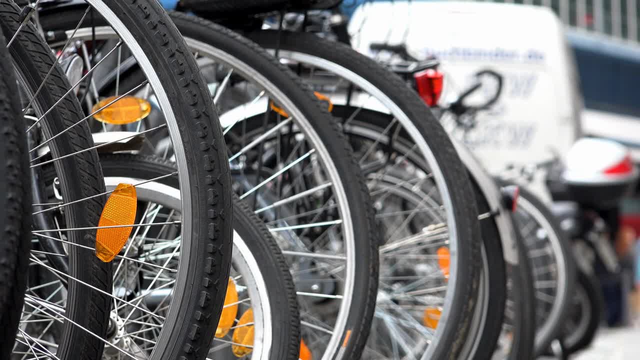 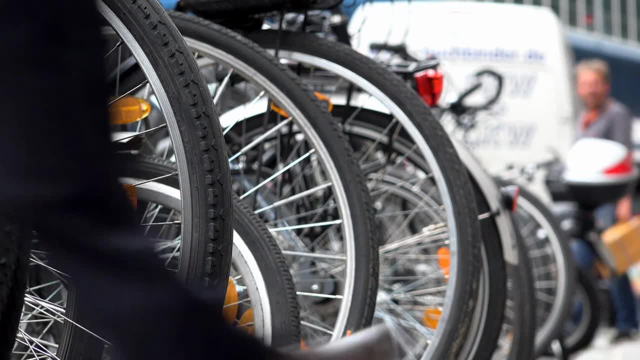 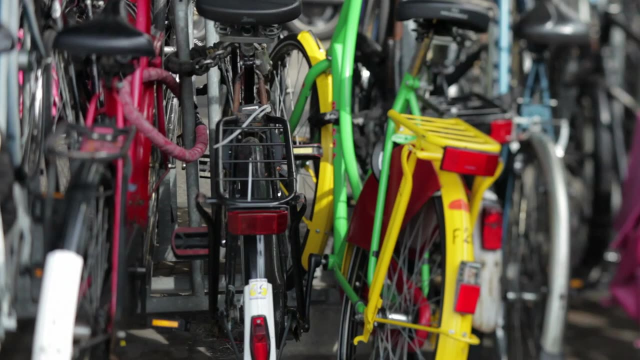 This means no chance for accidents. 3. Minimize Raw Material Consumption and Disposal. 4. Reduce the Risk of Injury to Passengers. 5. Sustainable Transportation Leads to Less Congestion on the Roads. 6. Reduce the Risk of Accidents. 7.. 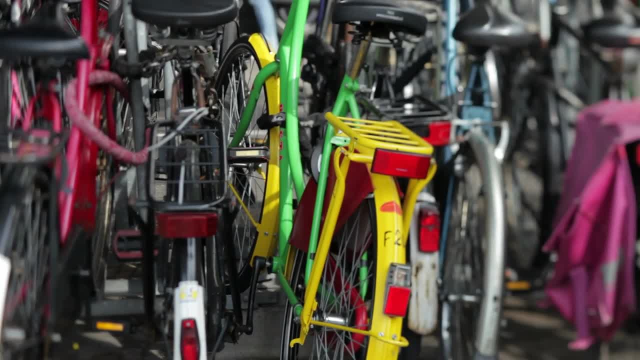 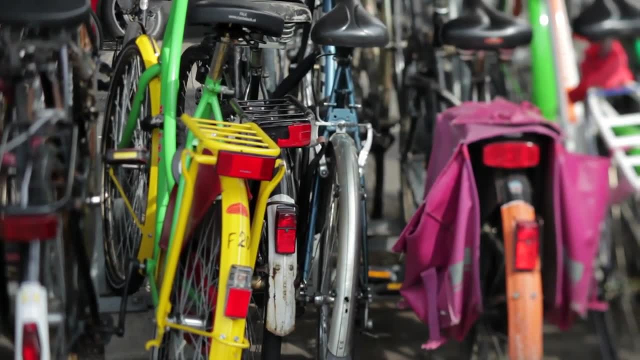 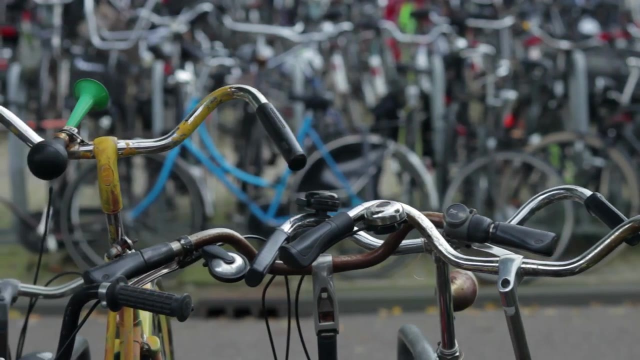 Minimize Noise Pollution. 8. Increased Safety Due to Reduced Risks and Potentials for Collisions. How to Get Started with Sustainable Transport? Whether you're a driver, passenger or pedestrian, the first thing to do understands your needs and find ways to meet them. 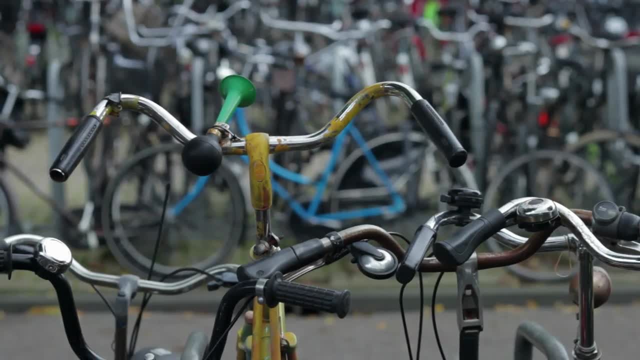 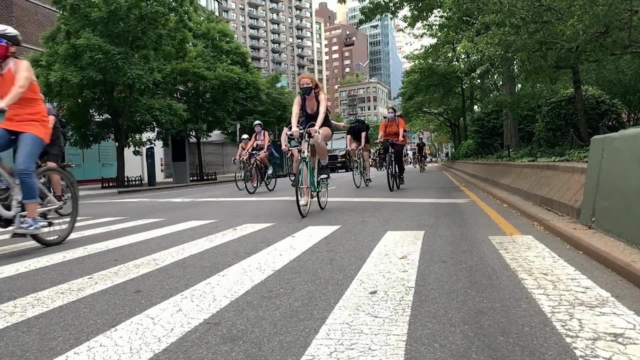 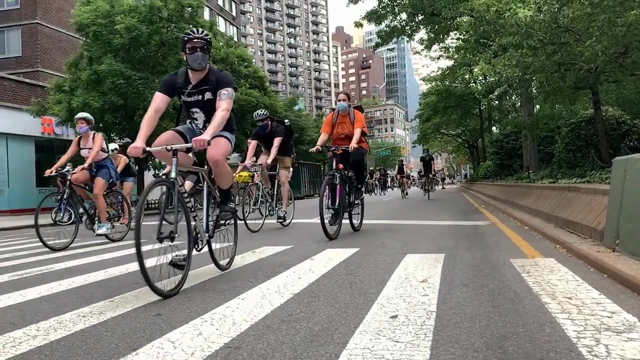 For example, one way transportation can be made sustainable for everyone is through carpooling. This strategy reduces congestion on roads, decreases emissions of greenhouse gases per person and saves money. Other options include cycling more often, using public transport if possible, and walking. 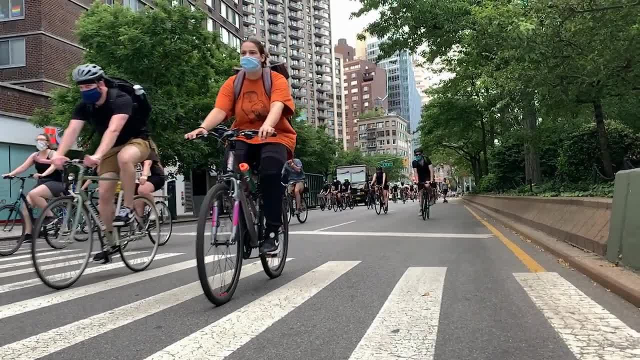 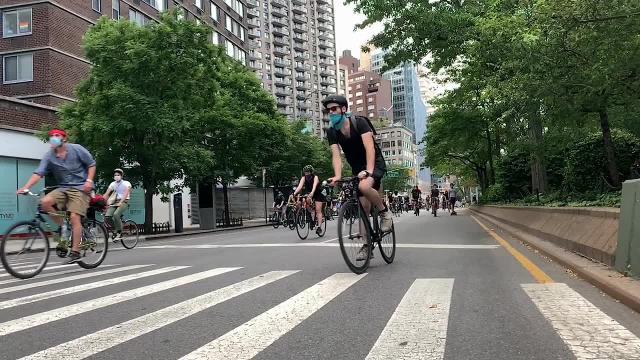 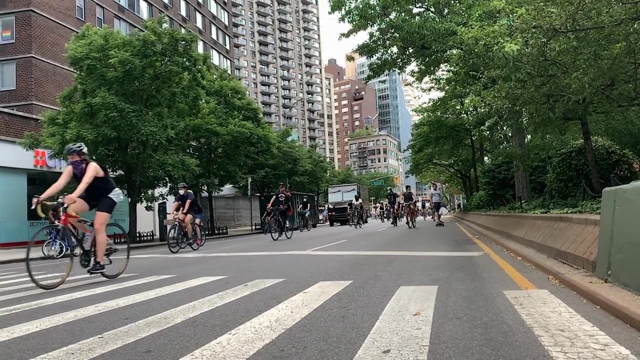 as much as possible when not driving 1.. If you have found that these are no longer viable solutions, it may be time to start looking into electric cars. Electric cars emit fewer GHGs than their petrol counterparts. In addition, they are cheaper over the long term, because electricity costs half of fuel. 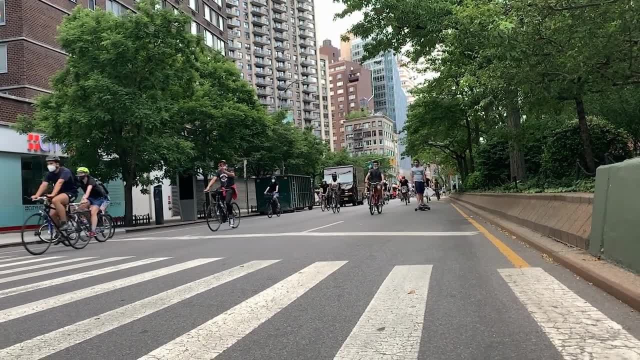 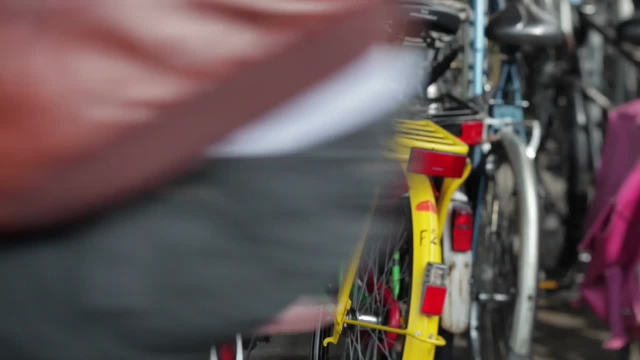 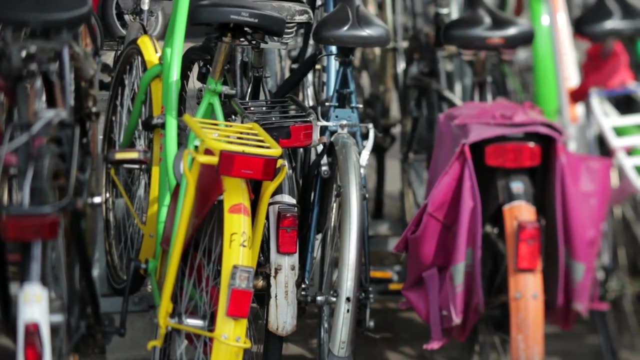 with an average range of 200 miles. 2. Ride with Friends When You Can Try carpooling with coworkers. 3. Cycling or walking whenever possible is a great way to reduce your carbon footprint and help the environment. It also benefits you by reducing stress levels, lowering the risk of diabetes and heart disease. 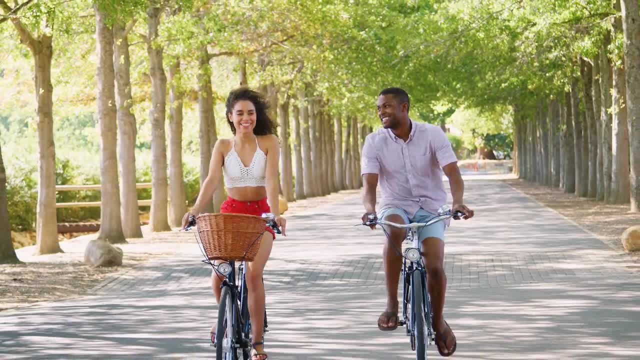 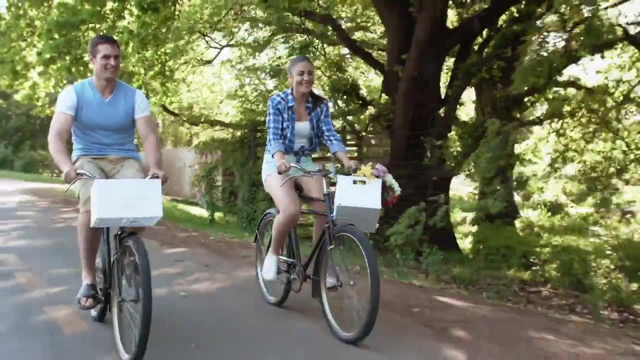 Options for sustainable transportation are available now, but we will need new technologies in the future to make it truly sustainable. Transportation currently accounts for 25% of GHGs emitted globally. This number must be decreased if global warming is going to stop, and we are not able to do. 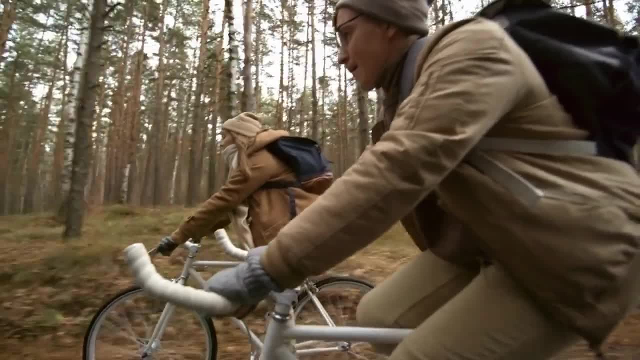 anything about it. With the latest news, the US Department of Health and Human Services has announced a new plan to stop global warming by reducing GHGs in Europe. It also includes a new approach to environmental disasters, such as hurricanes, from becoming worse. No matter what mode of transport you use, there are ways in which you can make it more. 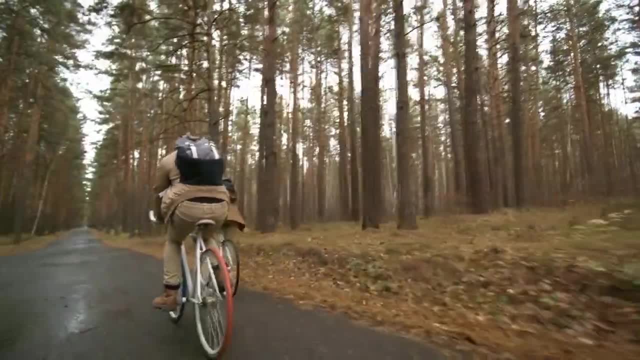 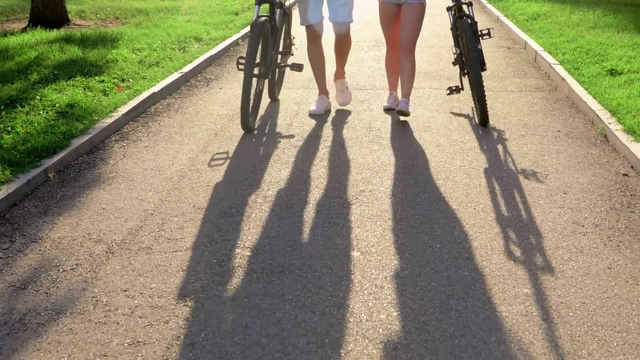 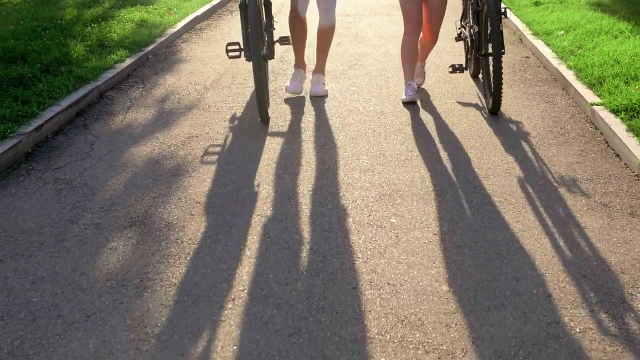 environmentally friendly, while benefiting yourself too. One option is using electric cars. Showcase what life could be like if everyone was on a bike or in a car that runs on clean energy. The future of sustainable transportation starts with the people. What if everyone could bike to work? 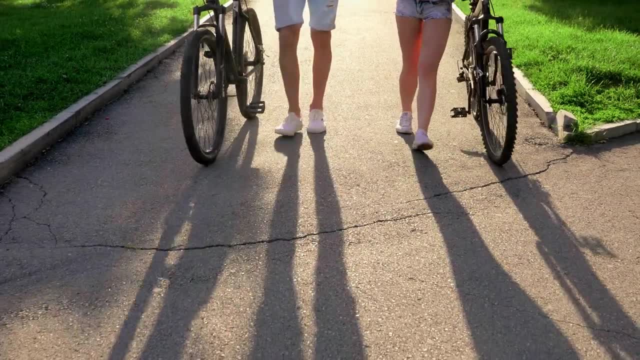 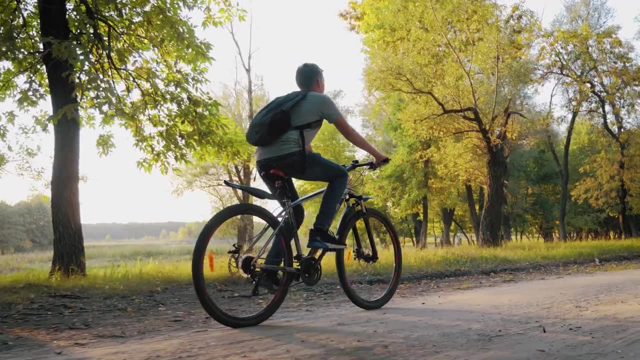 Or what if we all had electric cars that could help us, electric cars that ran on clean energy like wind or solar power. This post will explore how these changes might affect our lives for the better. In this future-focused world, bicycles would be a popular form of transit. 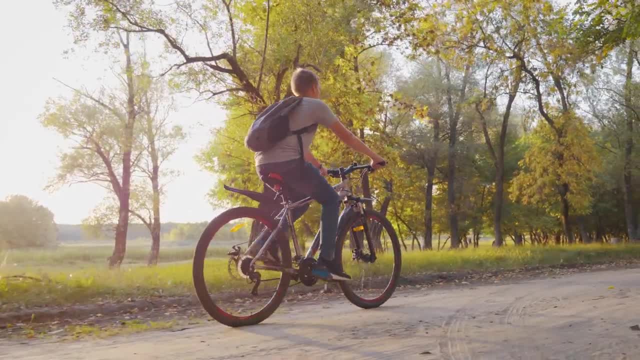 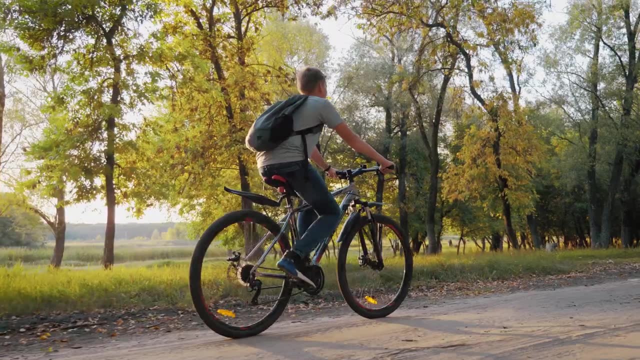 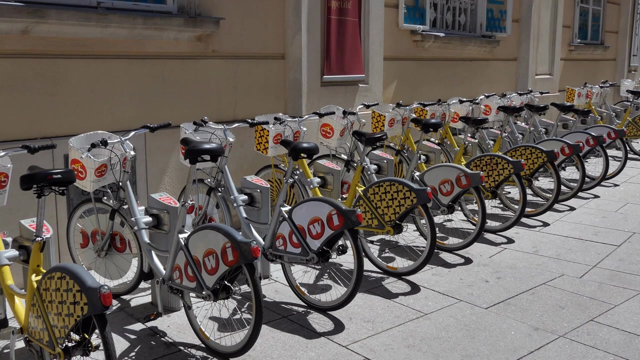 People who live in cities and other close-in areas would pedal their way around town. In contrast, those living in more rural areas would have access to low-emission buses and trains powered by renewable sources like wind turbines or solar panels. Electric vehicles- EVs- running on renewable energy are predicted to be commonplace as 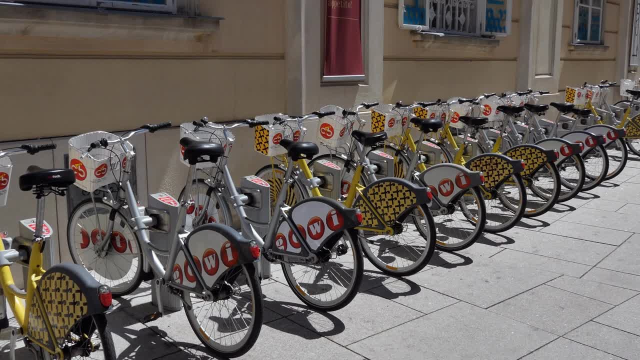 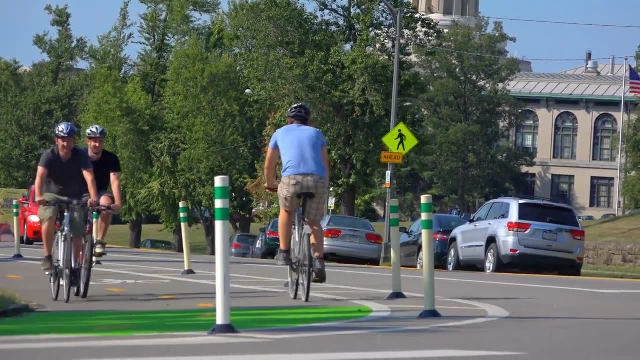 well. they'll help reduce greenhouse gas emissions just about everywhere. Low cost, clean energy is a future that we can't wait for. A world with fewer cars and more bikes will be healthier, not only because of the cleaner air, but also because biking to work burns calories as well. 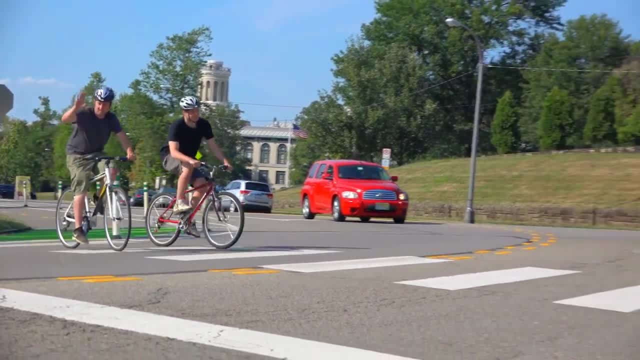 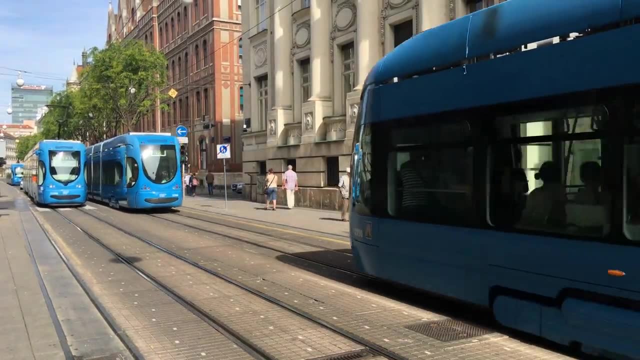 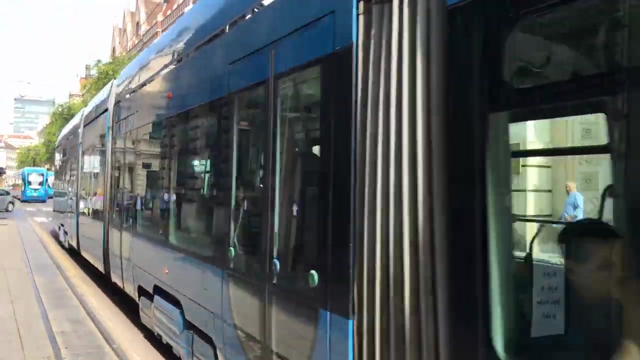 Studies show that people who live in walkable communities are happier too. there's nothing like fresh morning air to help you get started on your day. It may seem far away, But this sustainable transportation future feels right around the corner. Most Popular Sustainable Forms of Transport. For the longest time human beings have been. 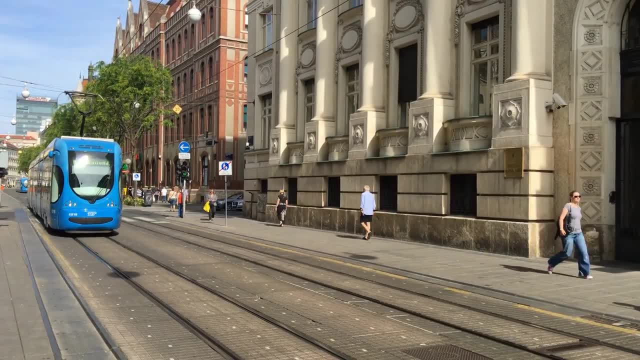 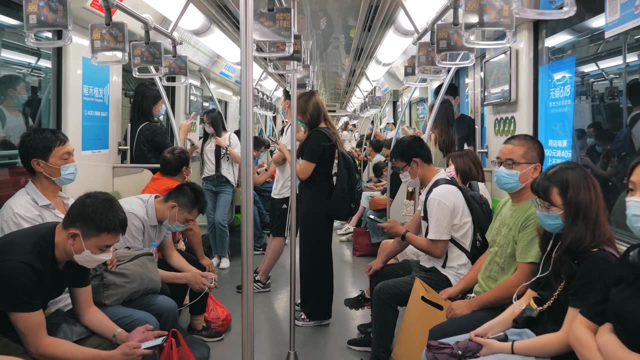 reliant on mechanized systems to get from one place to another These days, even with advances in technology, such as public transportation and cars, fossil fuels are still a huge part of how we travel around our cities and towns. Nowadays, though, there is an ever-growing number of people looking for a better life. 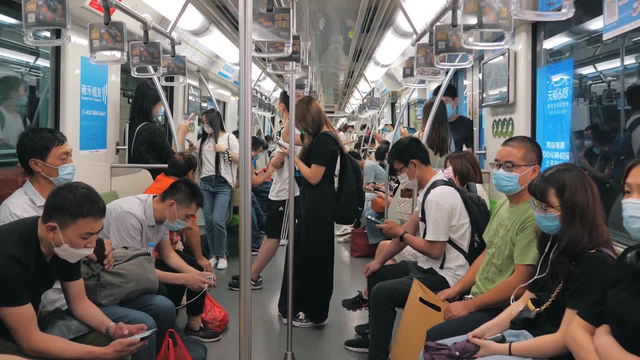 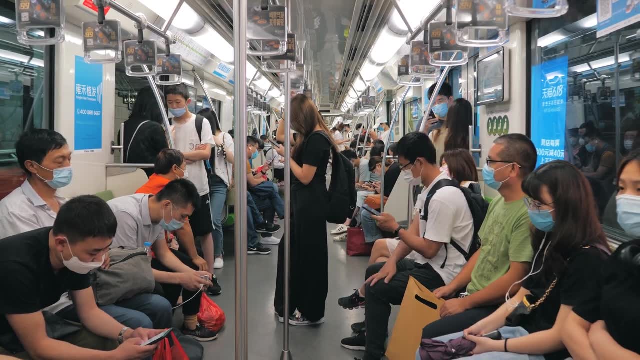 But there are still many who are not. There are many who are looking for ways to reduce their environmental impact by leaving their car at home or taking the bus instead. So, to be more eco-friendly and a better person for the planet, try these sustainable transportation. 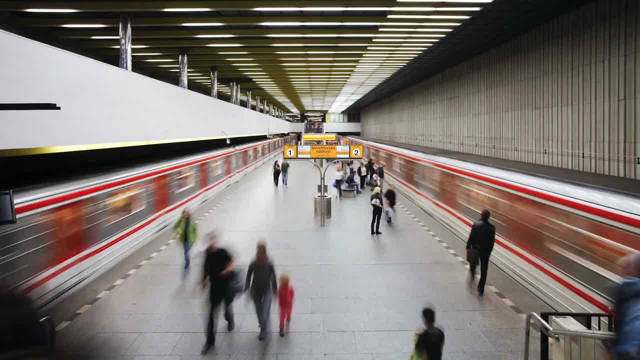 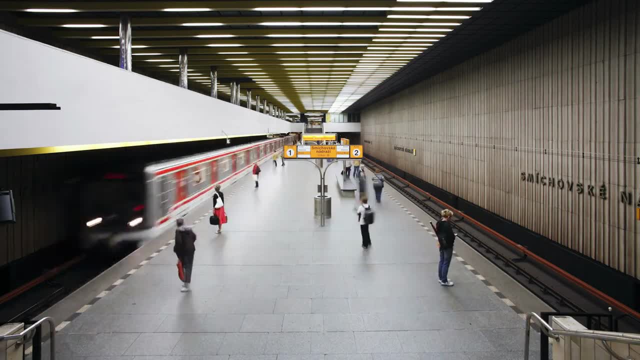 ideas: 1. Ride your bike or walk short distances and save gas by not using the car as often. 2. You can also get an environmentally friendly electric vehicle when you need a new one for yourself in the future, so make sure to consider that alternative next time around too. 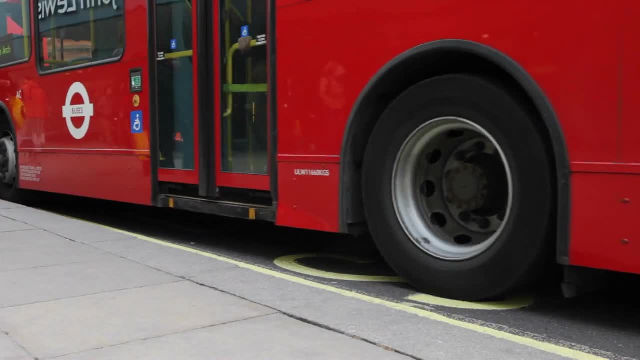 3. There's always public transportation. There's always public transportation. There's always public transportation, There's always private transportation, Because public transportation is an area of life. it's very easy to make your home a little bit more difficult. You're not going to get as much gas in your car as people do. 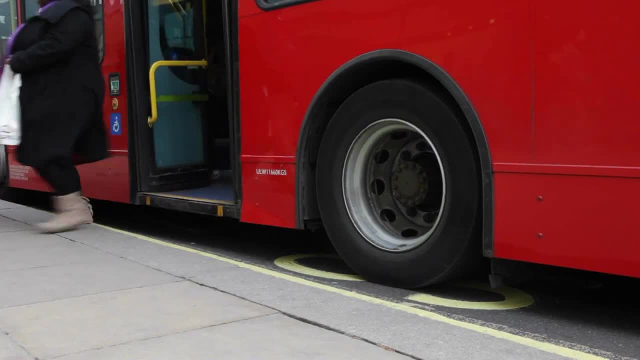 So if you're doing something like that, this is where you need to think about getting your car better, And if you're in a situation like this, be sure to keep some domestic transportation options available if they're feasible for where you live, which is another excellent 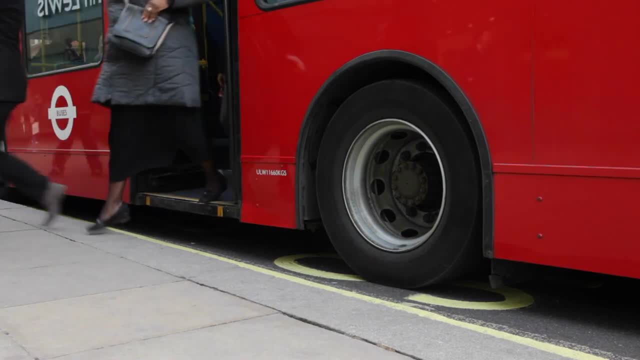 way of saving on gas costs while still getting from point A to point B, no matter what mode of transport. it may be, through safety-wise driving versus walking. I like these three tips because people should try their best at all times possible, just in case there will never be any more oil left out there. 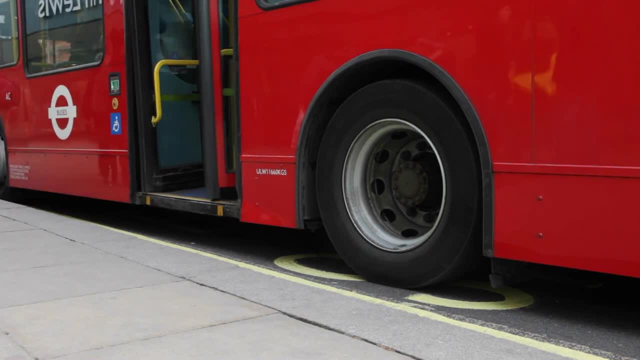 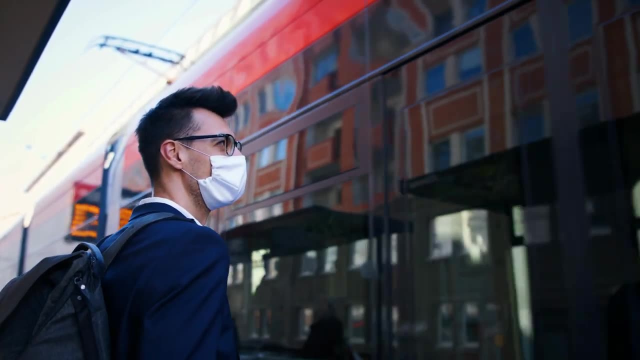 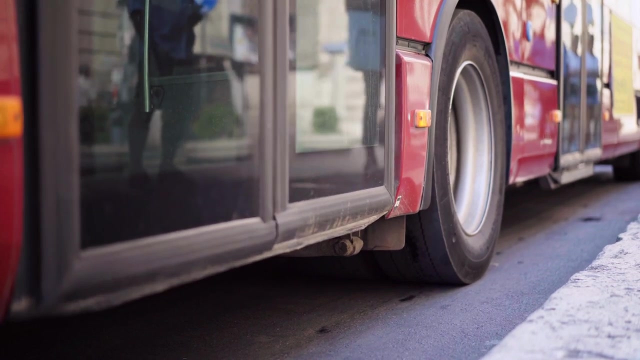 Benefits for employers who encourage employees to use sustainable transportation. 1. Increased productivity possible, just in case there will never be any more oil left out there. Benefits for employers who encourage employees to use sustainable transportation: 1. Increased productivity. Research suggests that employees who walk 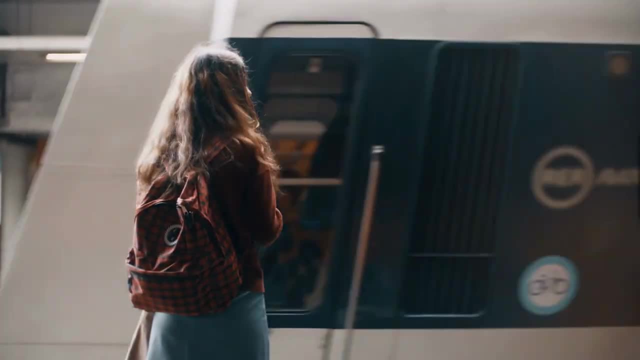 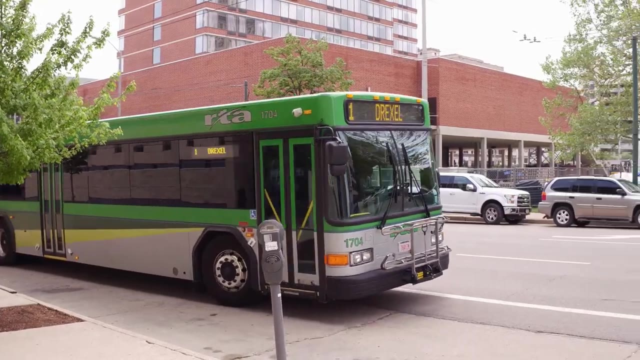 bike or take transit to work are more productive than their peers. 2. Reduced absenteeism and turnover rates. In a survey of 250 employers in 2010,, 17% reported they were facing increased absenteeism due to the lack of availability. 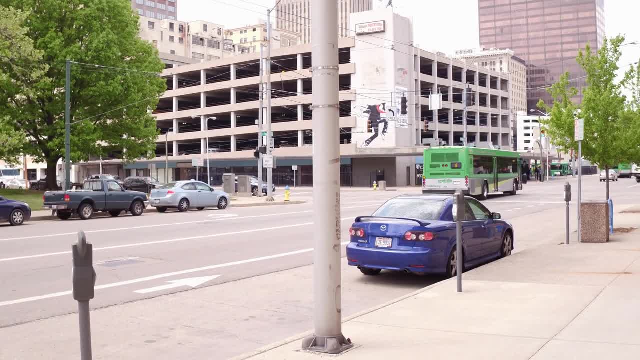 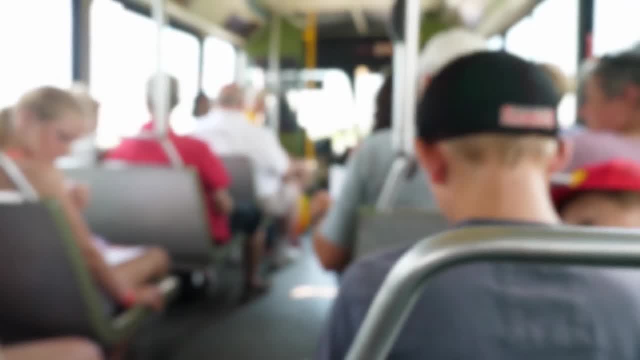 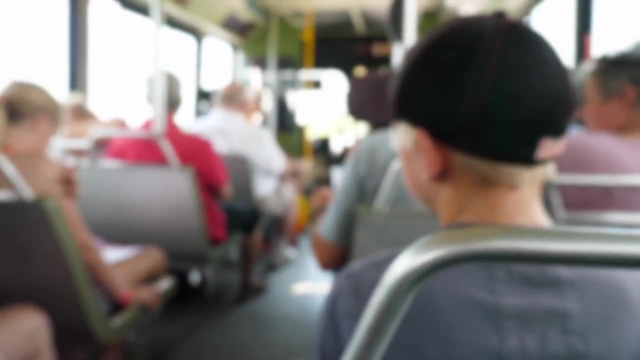 for public transportation. Studies have shown that if there is no viable alternative for getting to work, people will quit their jobs. 3. Employers also benefit from reduced fuel costs, which can be passed on to consumers as lower prices and improved economic performance through lowered gas consumption. 4. Safer environment. 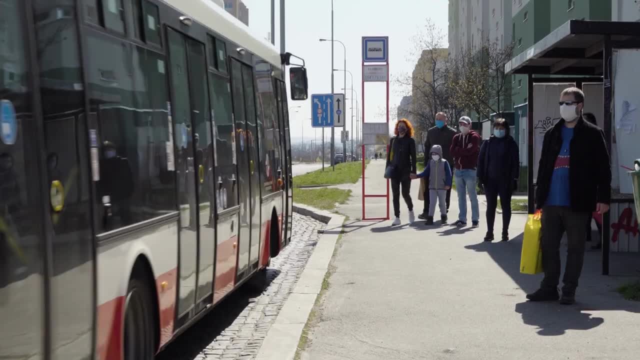 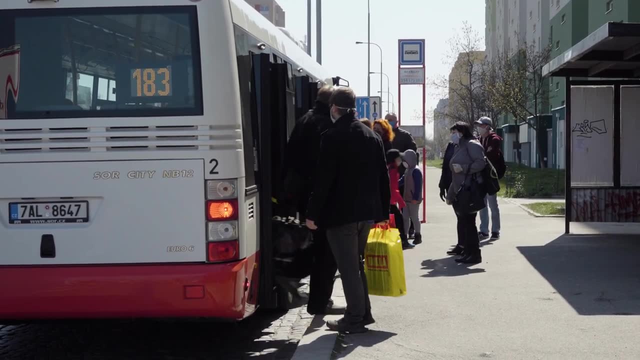 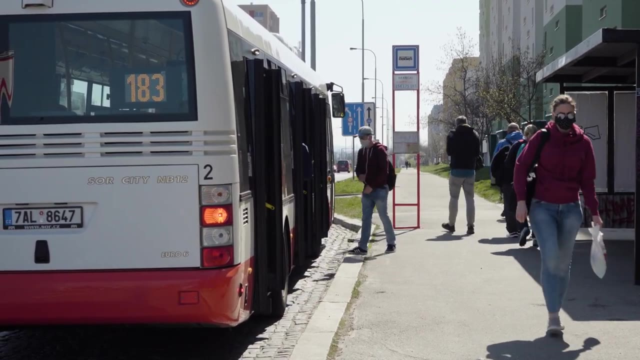 Employers should consider promoting sustainable transport options because it benefits the company's bottom line. 5. What it's like to live without fossil fuels and why we should all strive for this goal. The world is becoming more conscious of the importance of sustainable transportation. 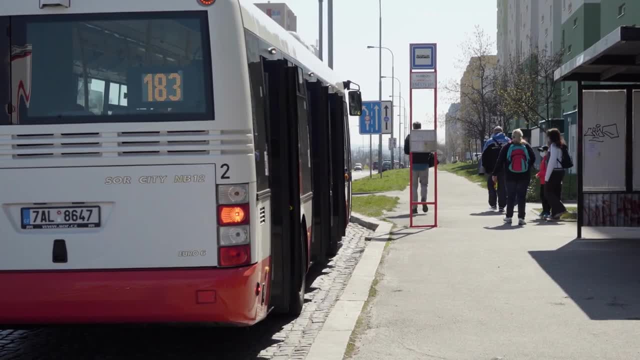 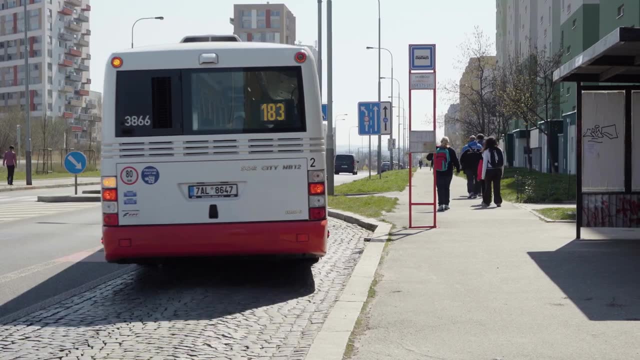 Every year, hundreds of millions of tons of carbon dioxide emissions are released into the atmosphere to power our modern society and economy. Choosing whether or not you want your future family to be affected by this pollution is a very important decision that needs to be made for us all to achieve sustainability. 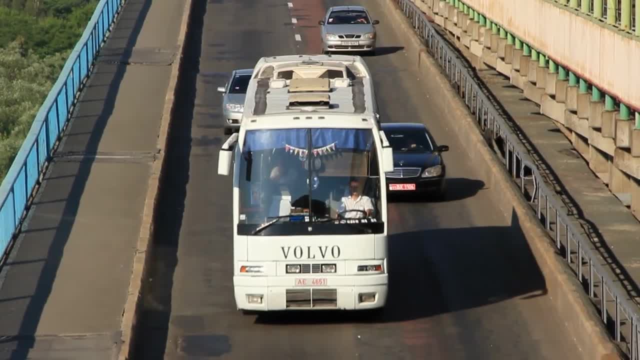 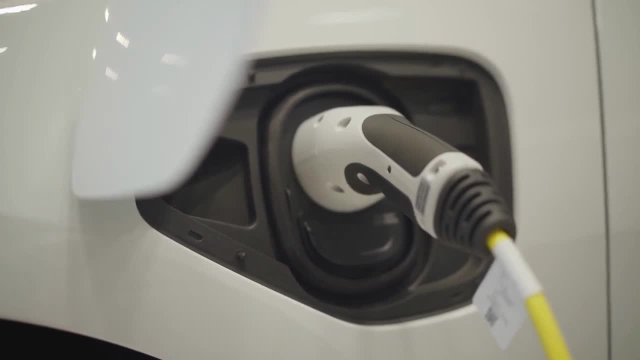 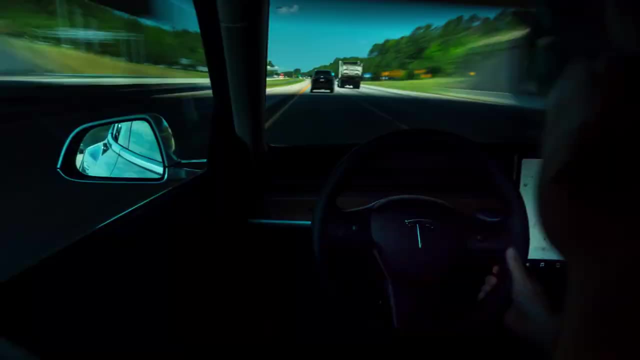 rar ajuste quality goals. fossil fuels will run out eventually and we need an alternative energy source before then. renewable energies such as solar power can provide affordable solutions for today's problems, while also providing long-term benefits through decreased dependency on fossil fuels. in addition, the global community should 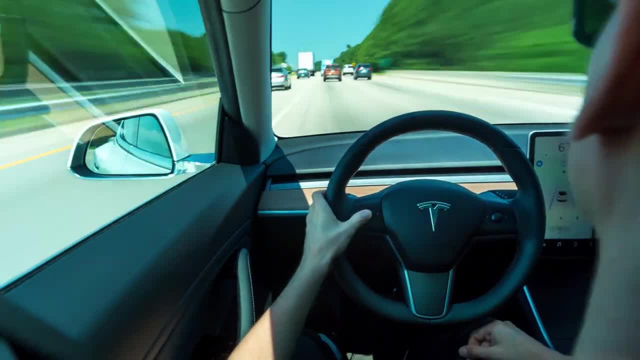 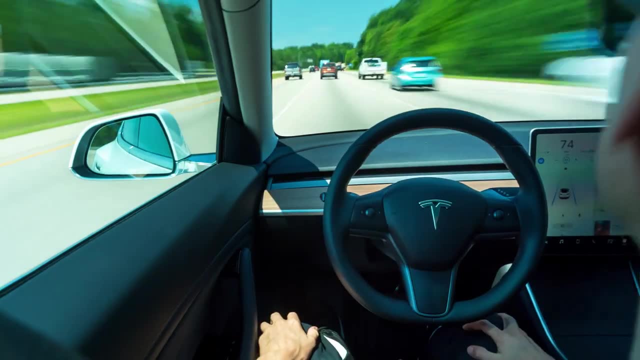 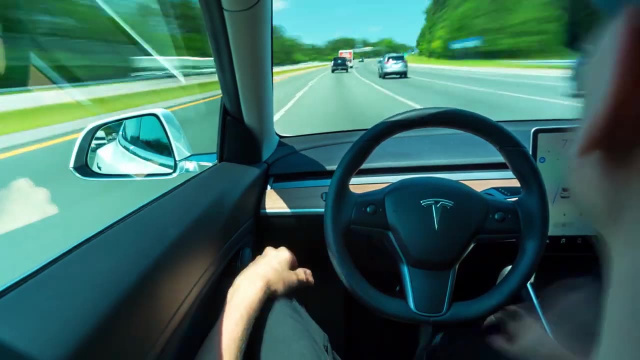 implement eco-friendly initiatives at home, like getting rid of gas-powered cars and air condition and many more things. the transportation sector is the largest and fastest growing consumer of fossil fuels. The world consumes 98 million barrels per day, accounting for 26% of all energy resources consumed globally. 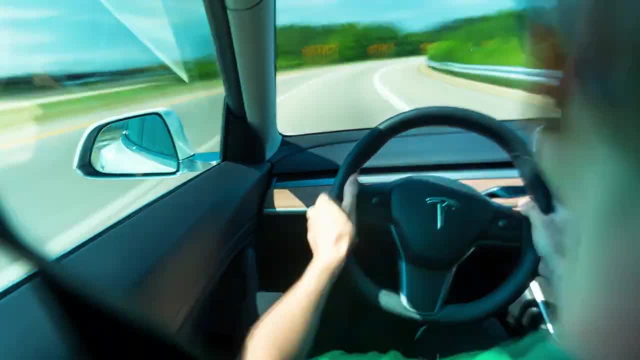 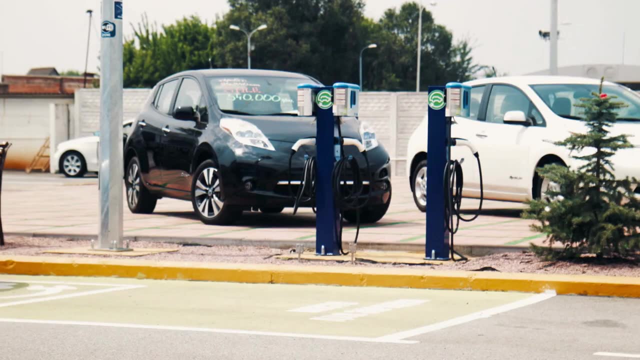 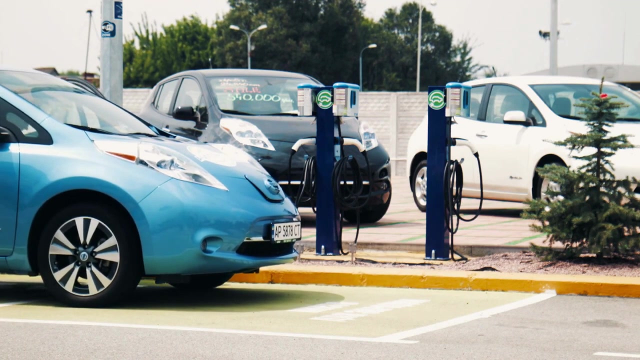 Transportation causes around 90% of air pollution in urban centers and 75% of global greenhouse gas emissions from personal vehicles are due to petroleum consumption. IEA Switching over to renewable power sources such as solar panels or wind turbines can provide affordable solutions for today's problems. 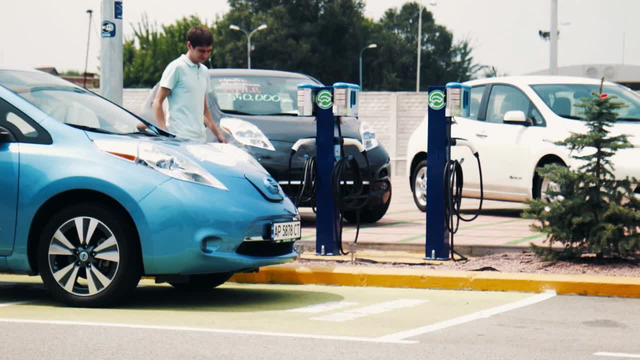 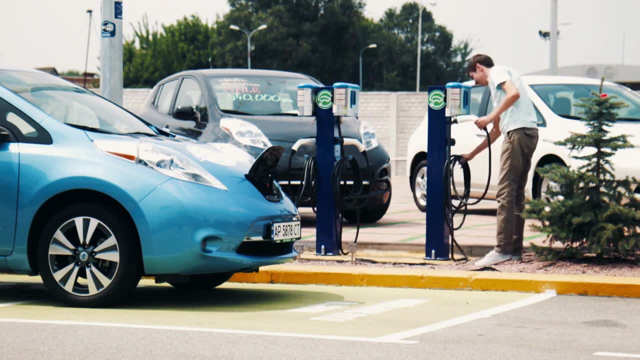 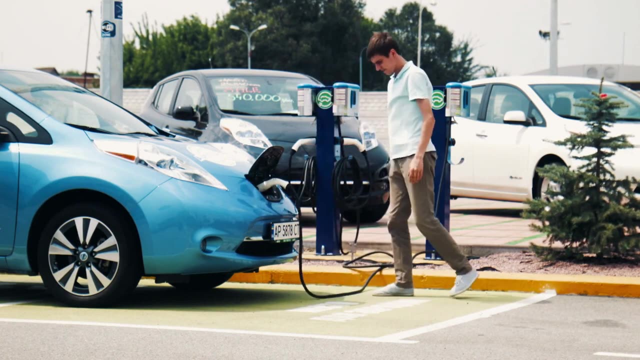 while also providing long-term benefits through decreased dependency on fossil fuels. Pollution caused by burning coal has been linked to cancer, asthma, stroke, heart disease and a host of other ailments like dementia. We need sustainable transport options now more than ever, because our future depends on sustainable, eco-friendly transportation. 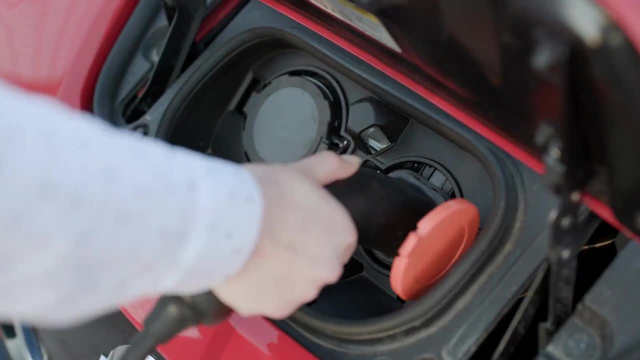 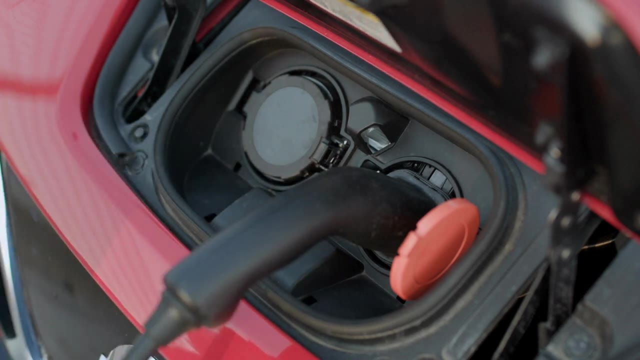 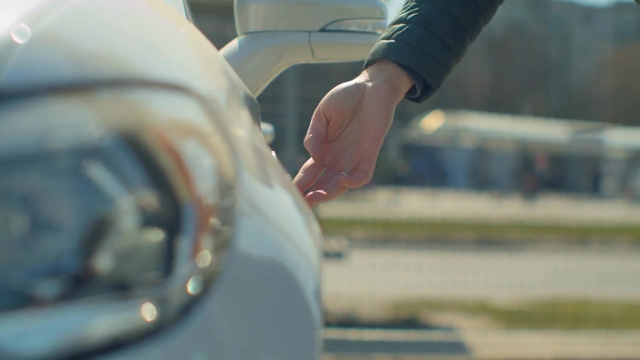 The future of sustainable transportation is a critical topic for the developing world, as it deals with pollution and poverty on an unprecedented scale. This article will provide information about how we can move towards sustainable transport solutions in our modern society, while also detailing some ways to make this process easier by creating urban centers that are more compact. 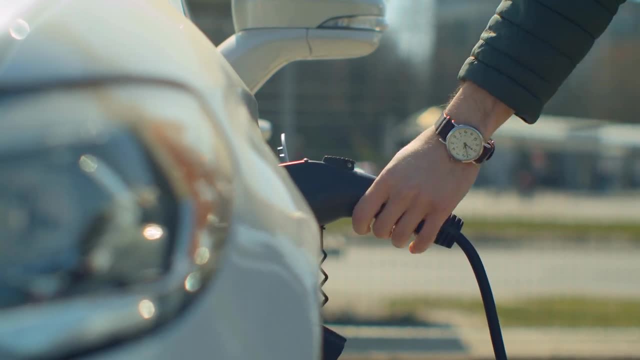 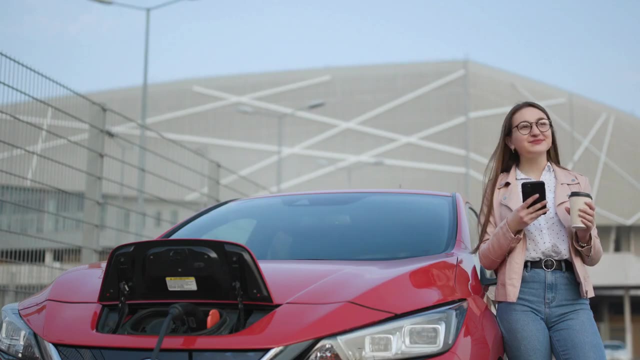 less reliant on individual personal cars and better connected through public transit or greenways, depending on the climate. Hopefully, these changes help combat current problems and create new opportunities as well, so that people have more access to jobs, services and resources, without having to travel vast distances or spend excessive amounts of time commuting. 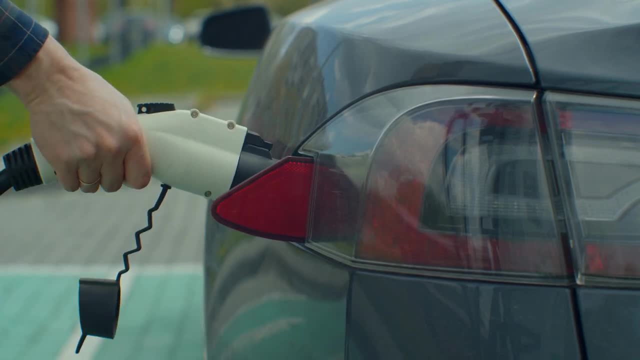 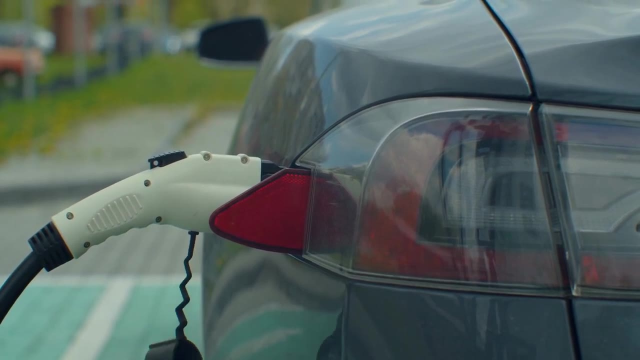 At last, it's time to start thinking about the future. The car is a thing of the past and it's time for you to get on board, or become obsolete, with your competition. Many benefits come with switching over from fossil fuel-powered cars, including better air quality in cities. 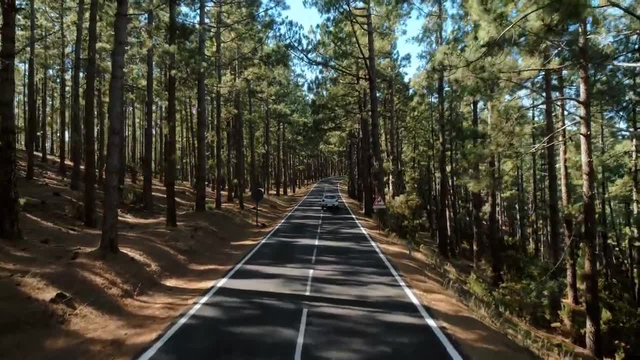 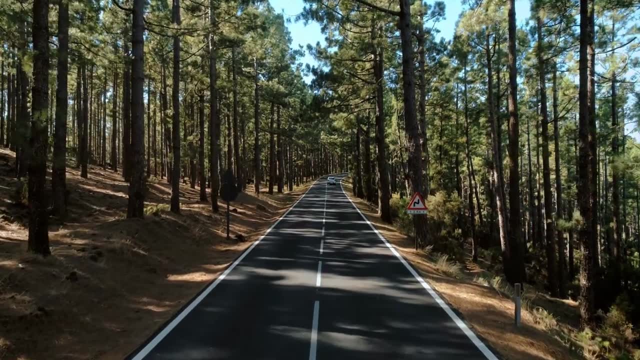 improved health outcomes due to less pollution exposure, reduced greenhouse gas emissions leading to lower global temperatures, and more money saved at the pump. For employers who want their employees to be happy while also helping save our planet, we offer solutions like EcoCarshare, which provides access to the world's most expensive cars.